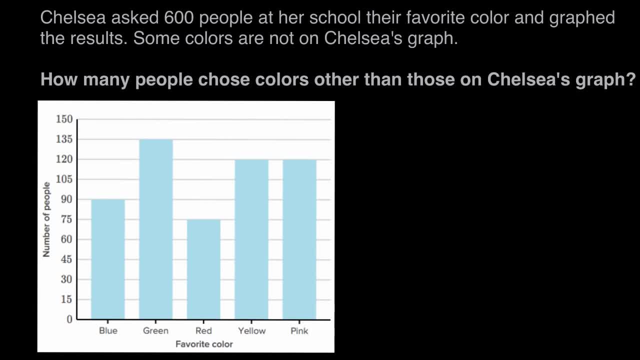 Chelsea asked 600 people at her school their favorite color and graphed the results. Some colors are not on Chelsea's graph. How many people chose colors other than those on Chelsea's graph? So here's Chelsea's graph. She made a bar graph and she listed some favorite colors. 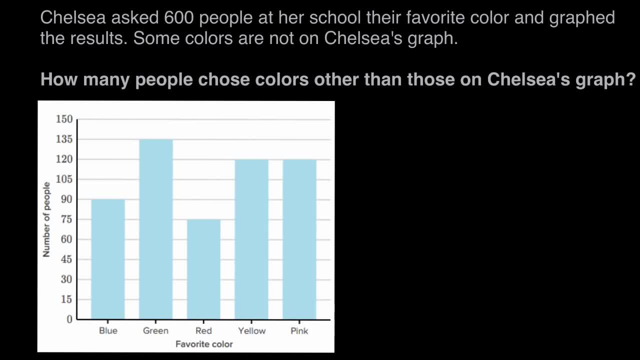 blue, green, red, yellow, pink and graphed people who had those favorite colors. But some of these 600 people like me had a different favorite color. My favorite color- orange- isn't on the graph, So we're asked how many people like me were not graphed. 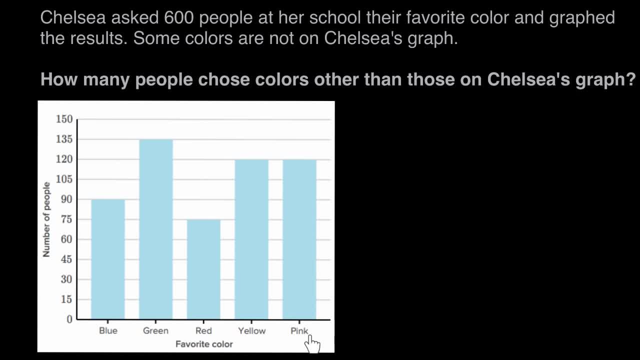 How many people picked a color besides blue, green, yet red, yellow and pink? So the way we can figure this out is if we look at the graph and figure out how many of the 600 people are on the graph, then we can take that away from the total 600 people. 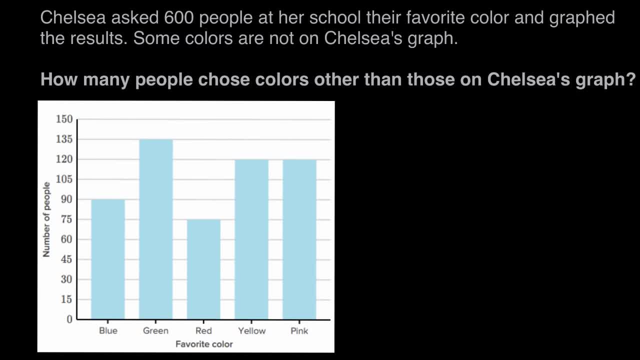 to find out how many are not on the graph. So we'll start by looking at the graph. First one, blue. This bar lines up to 90.. So 90 people picked blue Plus. next one green lines up to 135.. 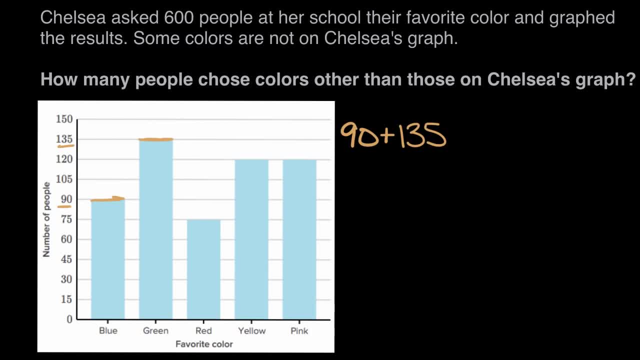 135 people picked green. Moving over to red, this bar lines up to 75.. 75 more picked red, Yellow and pink. the bars are the same heights. That means the same amount of people picked yellow and red. So let's go over and see that that was 120. 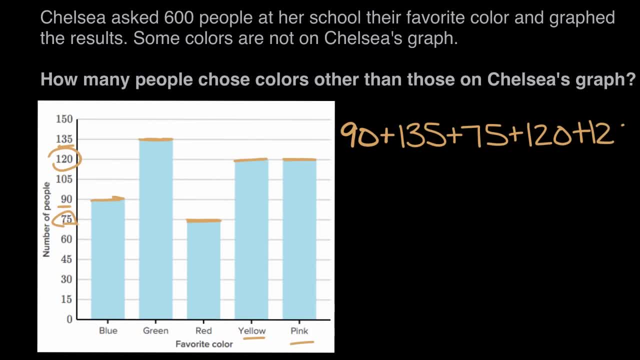 So 120 picked yellow and another 120 picked red. So if we combine all of these numbers, combine all the people that are on the graph, that will help us to figure out how many are not on the graph. So let's start with the ones. 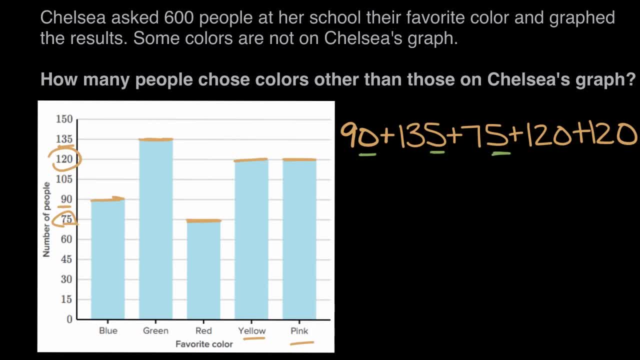 Zero ones plus five ones is five ones, Plus five more ones is 10.. Plus zero is still 10.. Plus zero is still 10.. So we have 10 ones Plus. let's look at our 10s, Nine, 10s plus three 10s is 12, 10s. 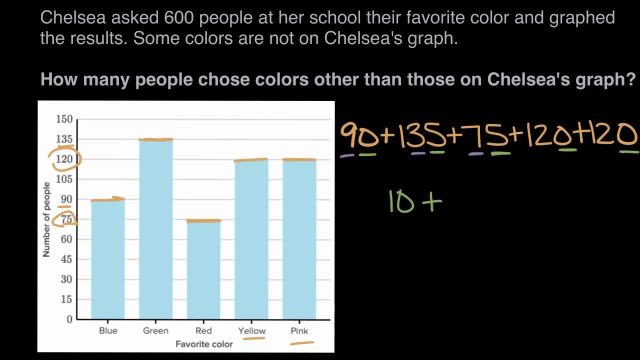 12 10s plus seven 10s is 19 10s. 19 10s plus two is 21 10s And two more 10s. 21 10s plus two more 10s is 23 10s. 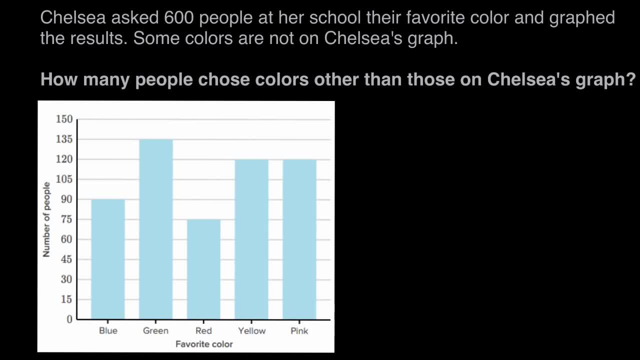 blue, green, red, yellow, pink and graphed people who had those favorite colors. But some of these 600 people like me had a different favorite color. My favorite color- orange- isn't on the graph, So we're asked how many people like me were not graphed. 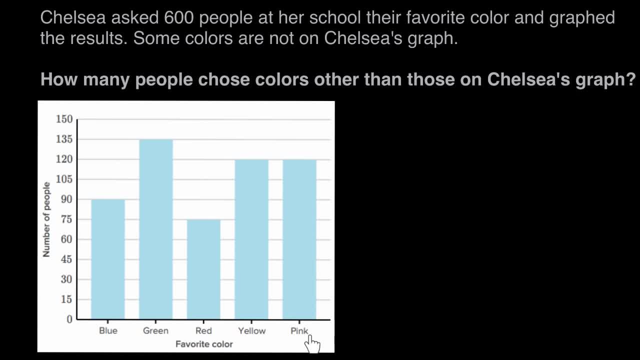 How many people picked a color besides blue, green, yet red, yellow and pink? So the way we can figure this out is if we look at the graph and figure out how many of the 600 people are on the graph, then we can take that away from the total 600 people. 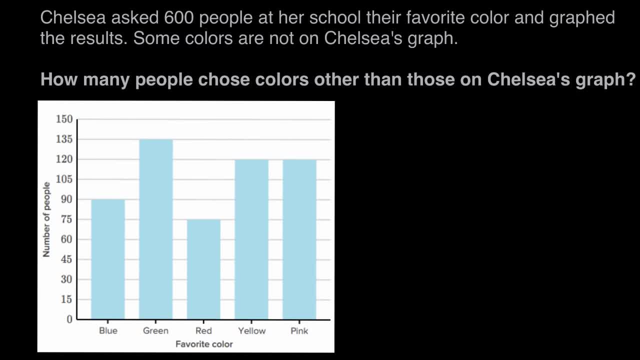 to find out how many are not on the graph. So we'll start by looking at the graph. First one, blue. This bar lines up to 90.. So 90 people picked blue Plus. next one green lines up to 135.. 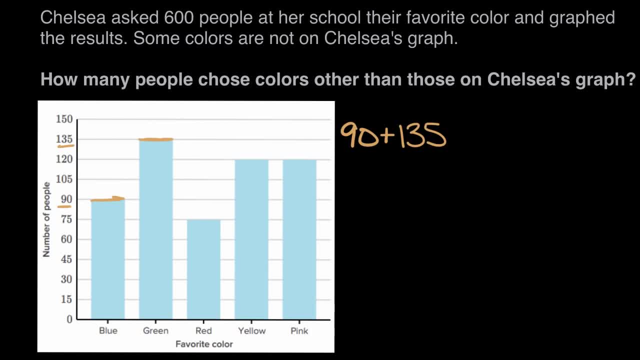 135 people picked green. Moving over to red, this bar lines up to 75.. 75 more picked red, Yellow and pink. the bars are the same heights. That means the same amount of people picked yellow and red. So let's go over and see that that was 120. 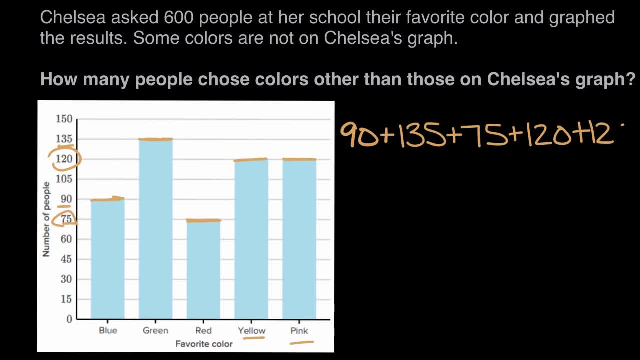 So 120 picked yellow and another 120 picked red. So if we combine all of these numbers, combine all the people that are on the graph, that will help us to figure out how many are not on the graph. So let's start with the ones. 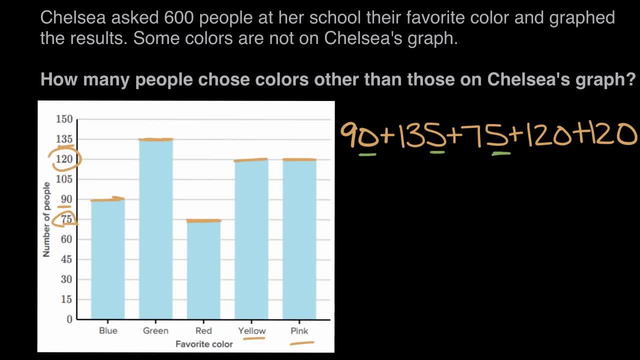 Zero ones plus five ones is five ones, Plus five more ones is 10.. Plus zero is still 10.. Plus zero is still 10.. So we have 10 ones Plus. let's look at our 10s, Nine, 10s plus three 10s is 12, 10s. 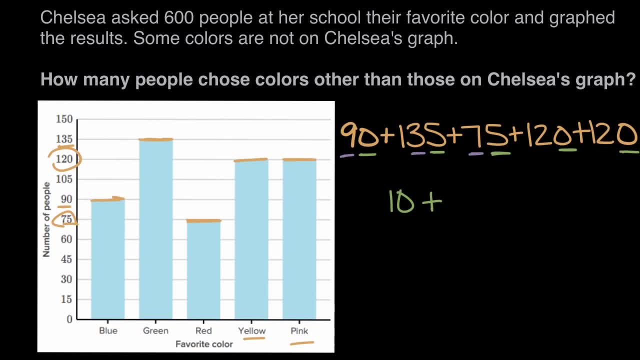 12 10s plus seven 10s is 19 10s. 19 10s plus two is 21 10s And two more 10s. 21 10s plus two more 10s is 23 10s. 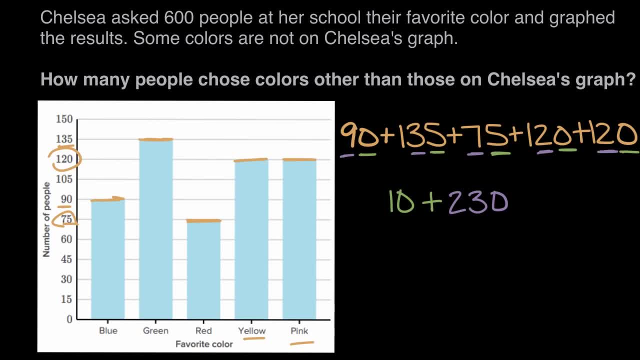 So we have 23, 10s or 230.. That's zero. so we're talking about 10s Plus. we can now do our 100s. Only a few of these had 100s. We had 100 plus another 100 is 200s.